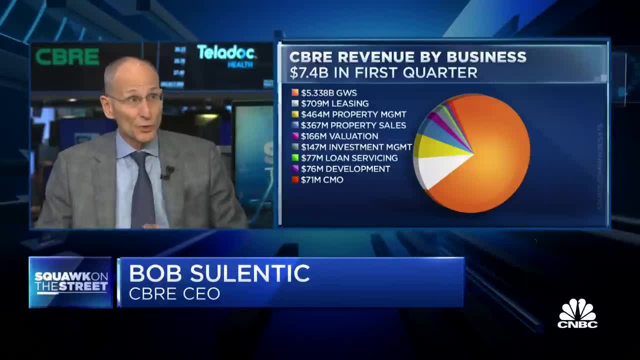 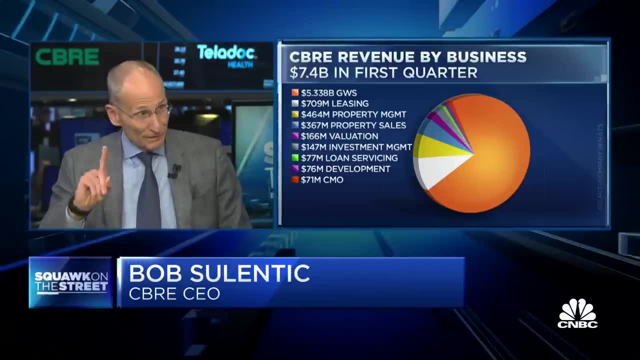 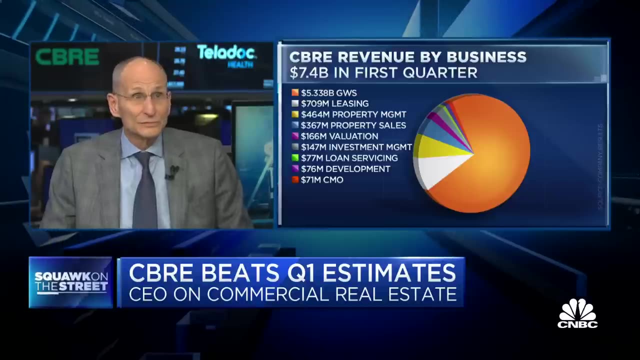 challenges in the banking sector associated with loans rolling over. But here's a statistic for you: About 1.5% of the balance sheet of commercial banks, 1.5% is in office assets. It's not going to be ruinous to the commercial banking sector. Yeah, it's only $80 billion. It's a big number. 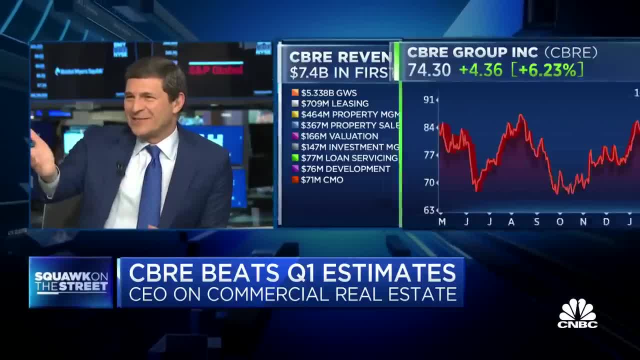 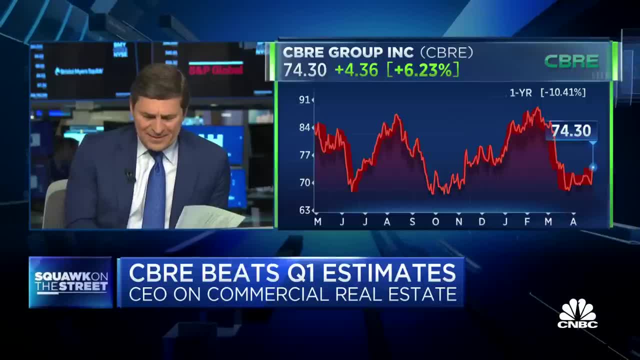 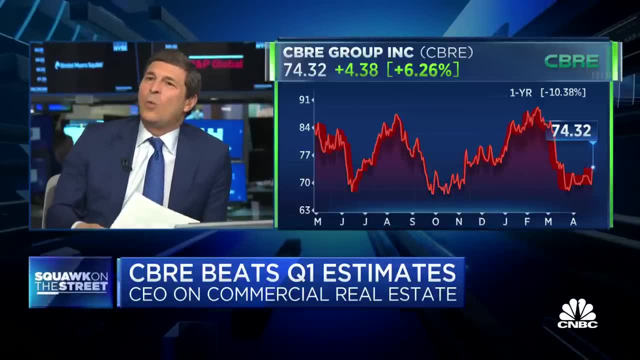 we all want to talk about it. I mean, and the Journal loves writing about it today, You know, there's this story about a building that was valued at $300 million a few years ago. It's going to sell for $60 million. You know what are the long-term implications here of the 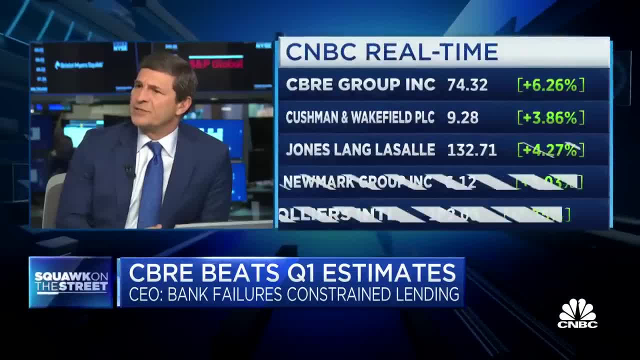 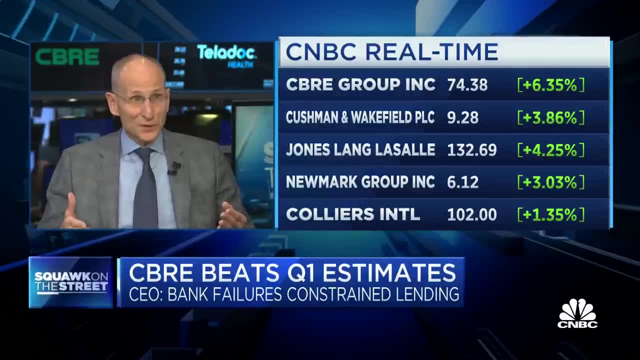 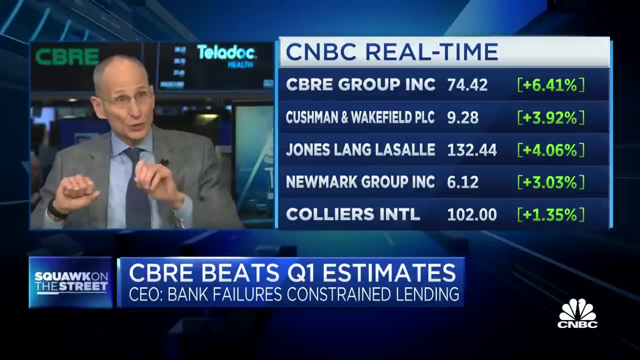 significant decline in values of some of these properties in major cities. David, there is going to be a decline in value for B and C office buildings, But what's going on with return to the office and challenges around return to the office is company. companies want their people back to a reasonable degree And the way they're getting that done is. 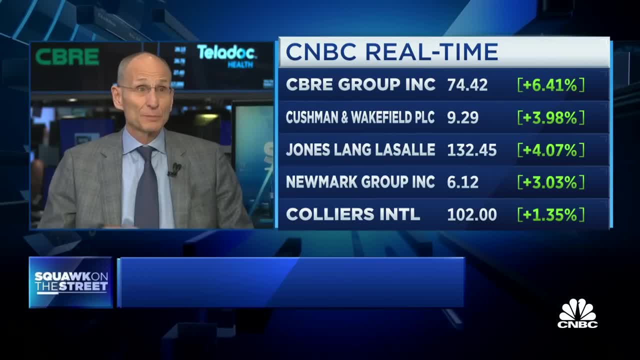 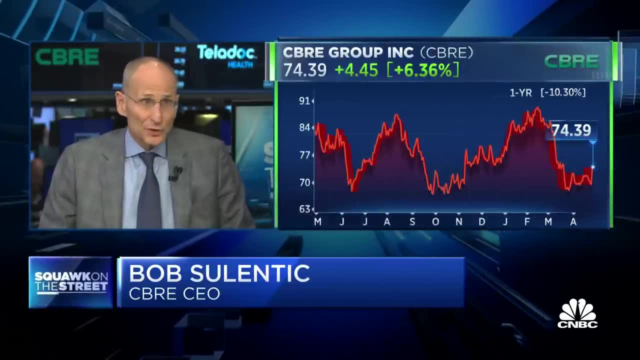 to create great office environments for their people. So the good office buildings, the A office buildings, the ones that are surrounded by amenities, with good infrastructure, those office buildings are still doing quite well. They're going to be valuable And while the office asset 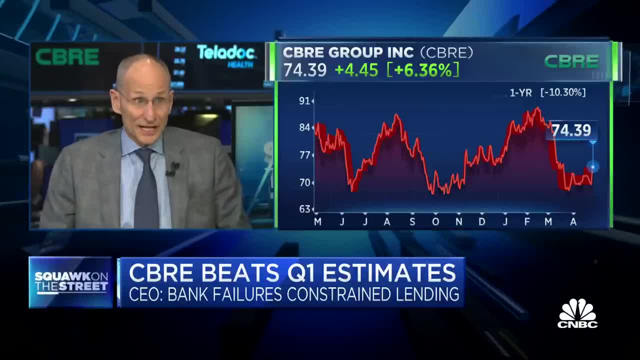 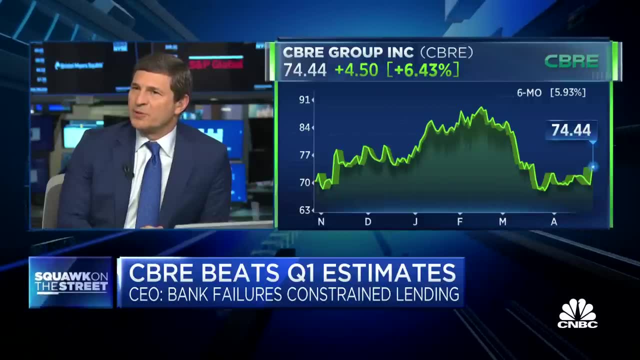 class is going to shrink, it's still going to be a very large asset class. You believe so. And what about this idea- that seems to be very difficult to accomplish in terms of the requirement of so much new capital- of converting buildings to residential 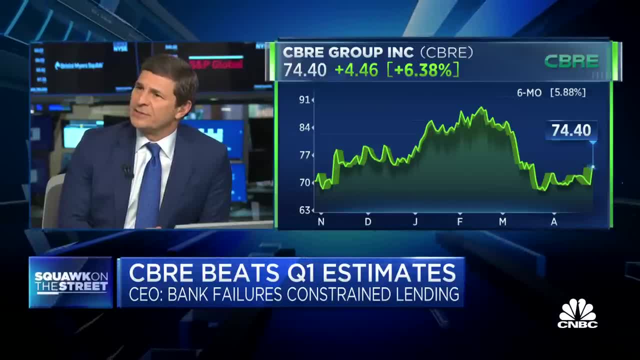 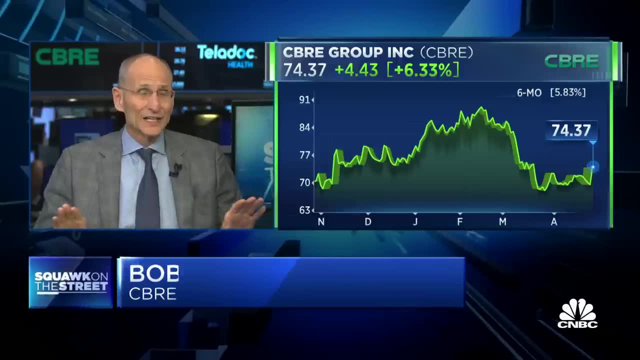 for example, given the need for housing in so many of these cities. Well, there is a big need for housing here in the US and around the world, and that's creating a real opportunity in commercial real estate. I think the opportunity. 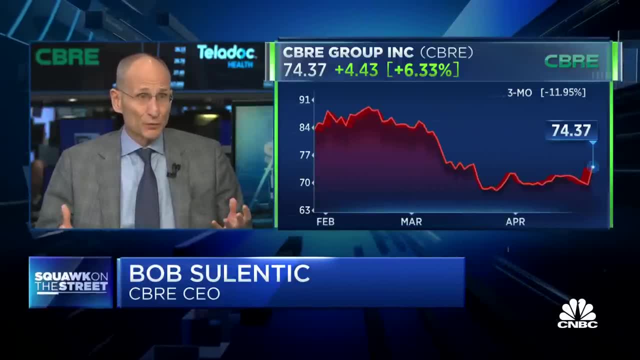 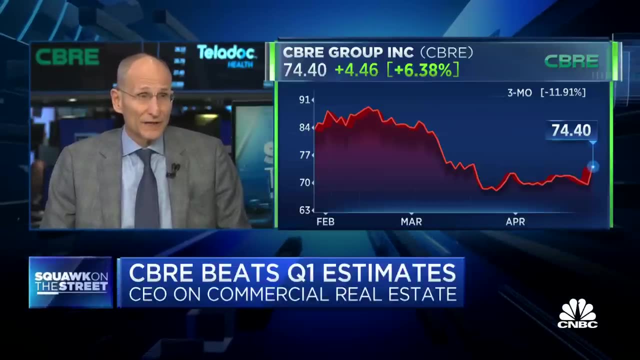 to convert a lot of these office buildings is going to be limited because the floor plates and the building infrastructure doesn't really effectively work for a multifamily residential. 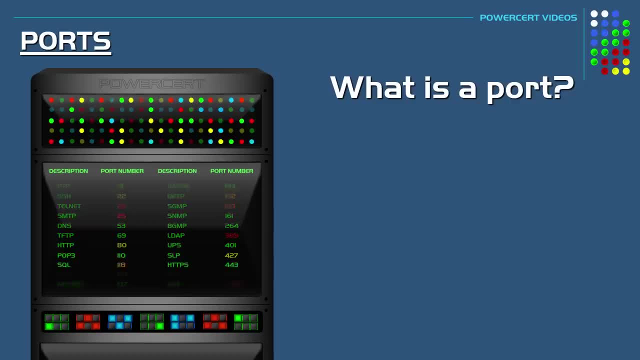 What is a port? So that is the topic of this video. Now. a port is not a physical connection. It's a logical connection that is used by programs and services to exchange information. It specifically determines which program or service on a computer or server that is going to be used.